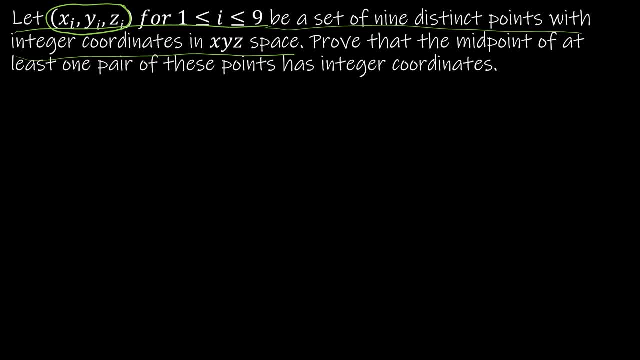 we have three ordered triples: X, I, Y, I, Z, I. This is just a numbering system. It's saying that there's nine distinct points. So, for instance, let's say I had a point zero, zero, zero, and I had a point one negative, two, three. 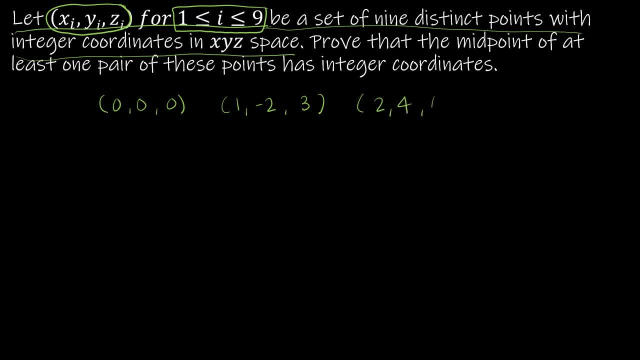 and two, four, six, you get the idea. I have nine distinct points, So none of the points are the same. This is just the first X, The first Y, the first Z. This is the second X, the second Y, the second Z, That's all this guy is. 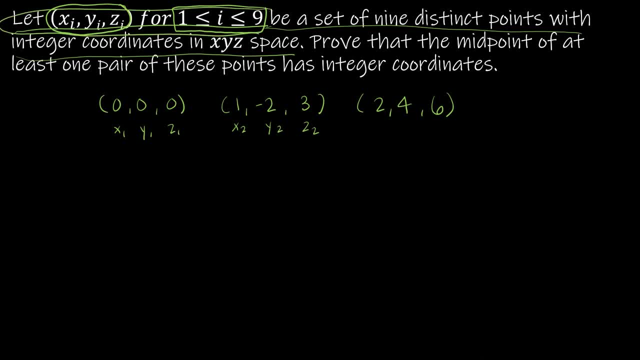 saying: Now again, we have nine distinct points. That's why it goes from one to nine, And they're integer coordinates on XYZ space. So again, they might have written it like that, or they might have said: where X, I, Y, I, Z, I? 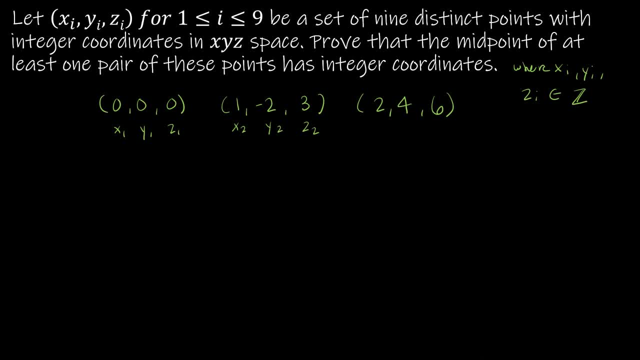 are integers. We want to prove that the midpoint of at least one pair of these points has integer coordinates. So we've talked about what all of this mess means, And now we need to talk about what does it mean to be a midpoint? So hopefully, again, you recall what it means to be a midpoint, But if you don't, 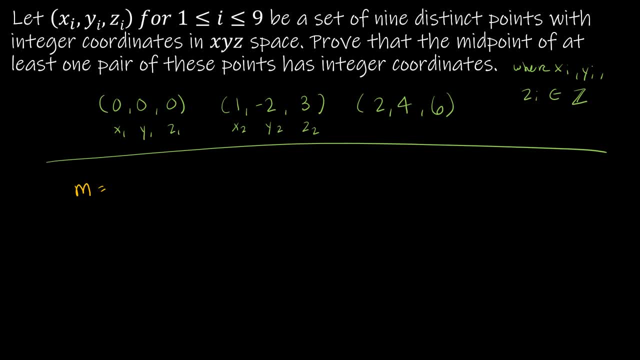 let's just remind ourselves: how do you define the midpoint? You can looking at these tables here you'll find the midpoints are the groups of the points where the points on Z and Y make up the number of points that match. So how would that make? 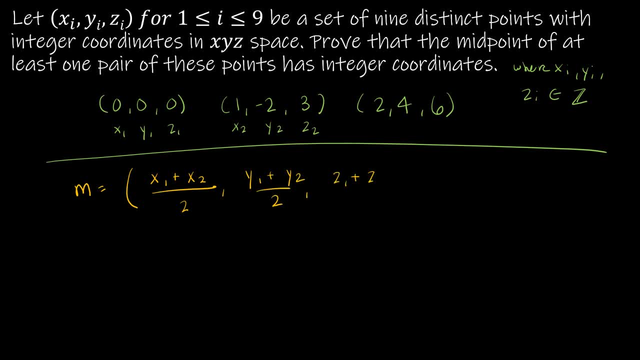 any sense. So this is something called the Poisson theorem. This is a simple equation using the Poisson theorem. The Poisson theorem is basically the following: You can see in this equation that you have two negative points. These are two positive points. 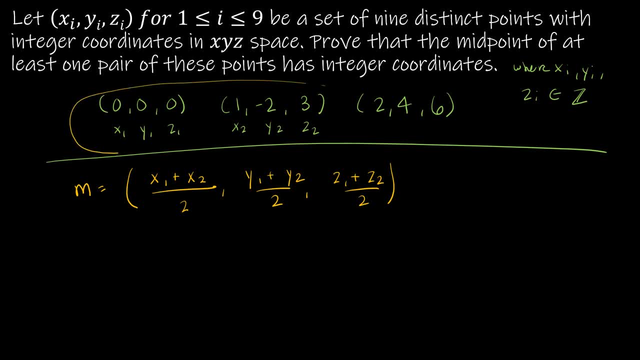 And one negative point is one zero And one positive point is one zero. These first two points that I made up my midpoint would be 0 plus 1 divided by 2,, 0 plus negative 2 divided by 2, and 0 plus 3 divided by 2, which would give me 1 half negative 1, and 3 halves. 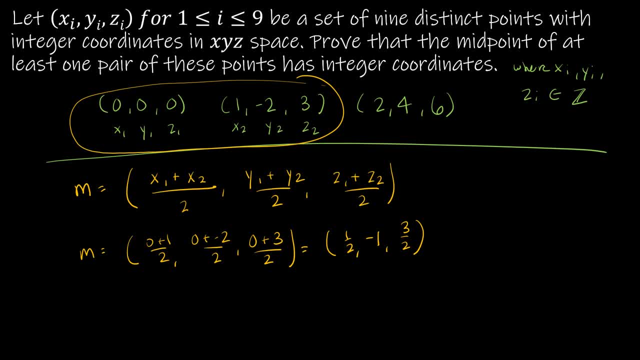 The last part of this says we want the midpoint of at least one pair of these points to have integer coordinates. So this example that I just did with you, not integer coordinates. So really I need it to be a member of Z Z Z, which it's not. 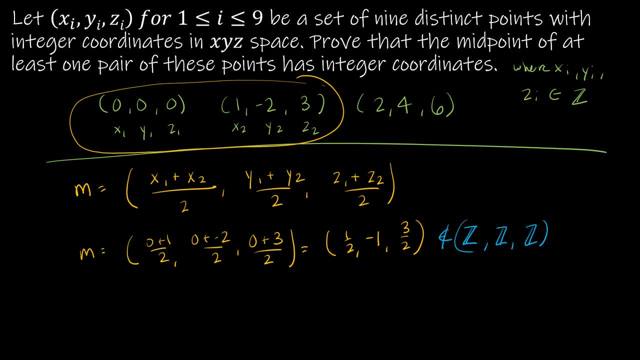 So how do I ensure that, when I add two things together and divide by 2, that the result is in fact an integer? Well, let's think about number theory. In number theory, which we studied, some in discrete math, 1,. 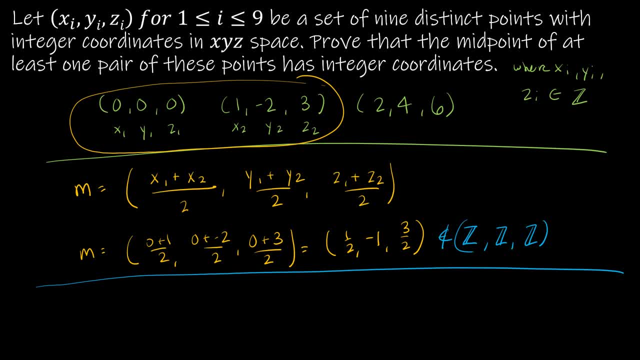 so I'm going to assume that you were joining us from discrete math 1, we showed that let's- and I'm not going to do a proof for any of these- We did these in discrete math 1, so just take my word for it. 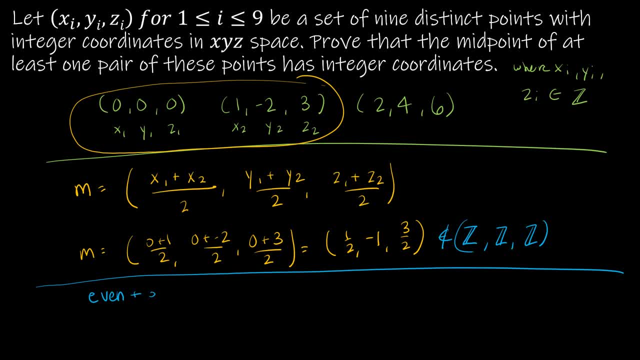 We found that if you take an even integer and an even integer- for example 2 plus 6, that that value is going to be even. And if I take an odd integer plus an odd integer- for example 3 plus 9,- 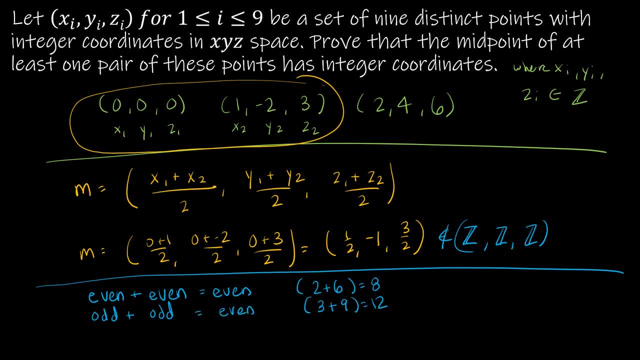 then that result is going to be even. But if I take an even plus an odd, like 2 plus 3, that solution is going to be odd, and that's in either order. So what do I need? Well, because I'm dividing by 2, I need my numerator to be even. 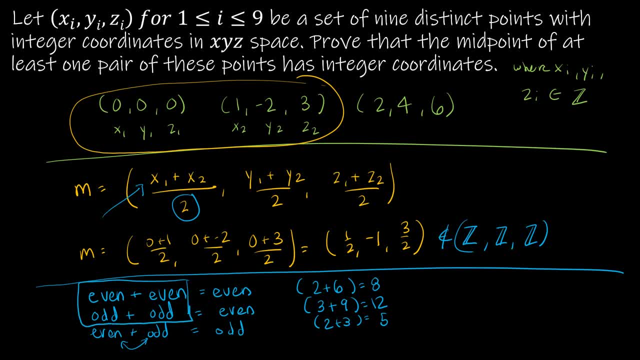 which means I need the two values- x1 and x2, and y1 and y2, and z1 and z2, to either both be even or both be odd. So the matrix is going to be even, And the mathy way to say this is that I need integers. 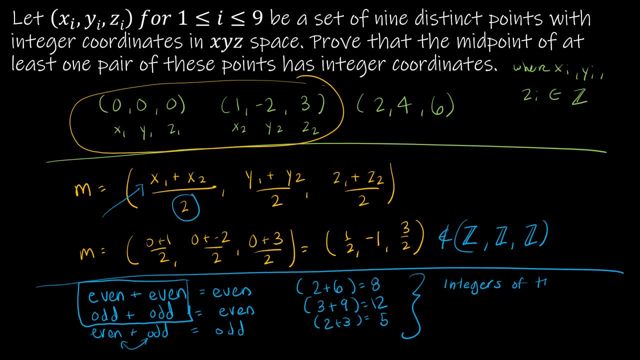 of the same parity. Parity talks about whether or not an integer is even or odd. So I haven't done the proof at all yet. All I have done is talk about what I need in order to successfully do this proof. So now we are going to essentially wipe our slate clean. 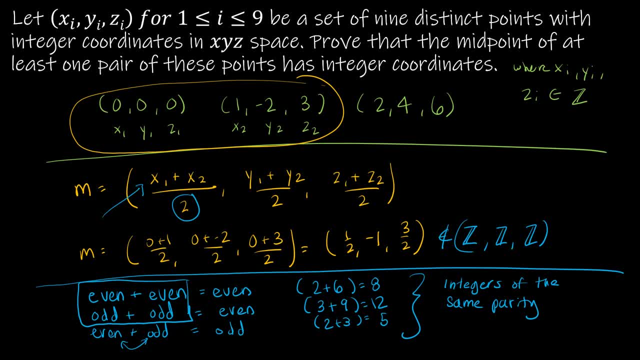 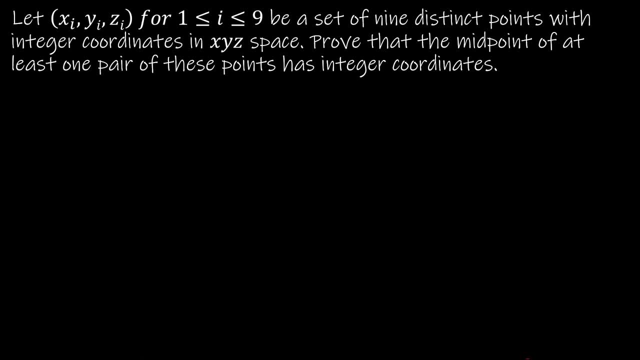 and go ahead and do this proof together. So now that we know how we are going to go about this proof, let's go ahead and prove it. So again, as we're working with the proof, it's a really good idea to structure your proof in a way. 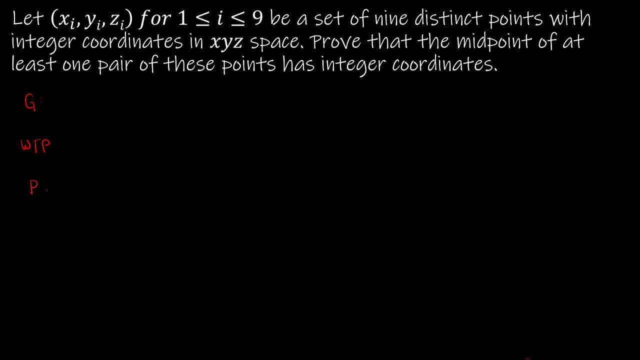 where you're going to have a given, a what to prove and a proof. I encourage my students to do that, just because it really helps us to know what is the information given to us. What's the premise? What are we trying to prove? 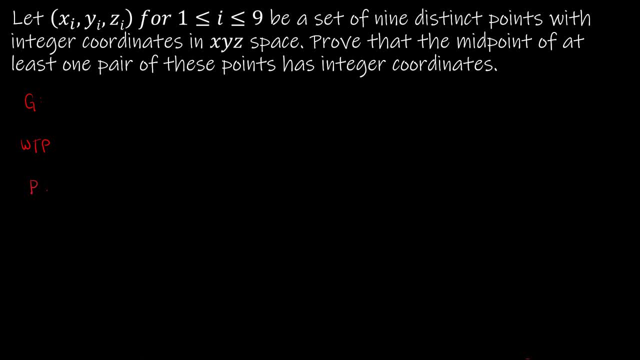 What are we trying to start with? Then the what to prove says exactly how we're going to prove it, based on our given and then our actual proof itself, And then the very last part, of course, will be our conclusion, which really should match the what to prove. 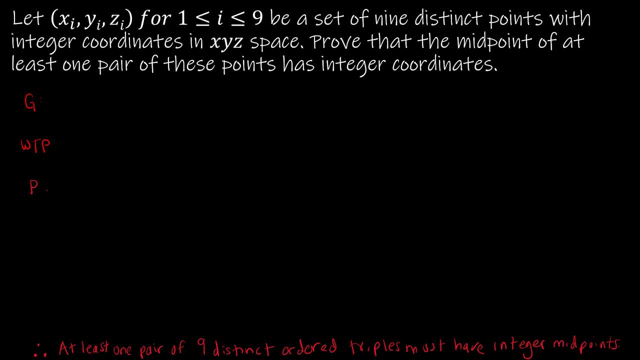 So in this case, I'm trying to prove that the midpoint of at least one pair of these nine points has integer coordinates. So for our given- we talked about the fact that it's really just that first sentence- We have an order, We have an ordered triple. 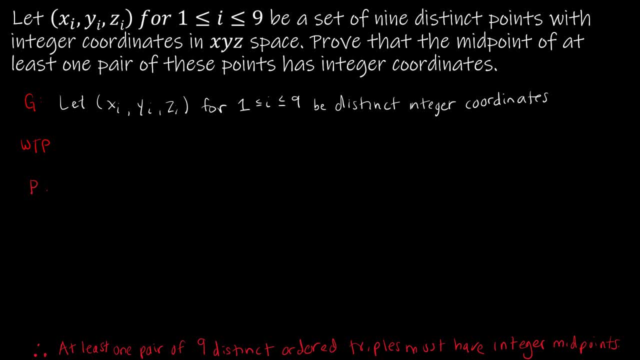 And we have actually nine of them. So for one is less than or equal to, i is less than or equal to nine, And they are distinct integer coordinates And what I'm trying to prove. I can either write what I wrote in red at the bottom: 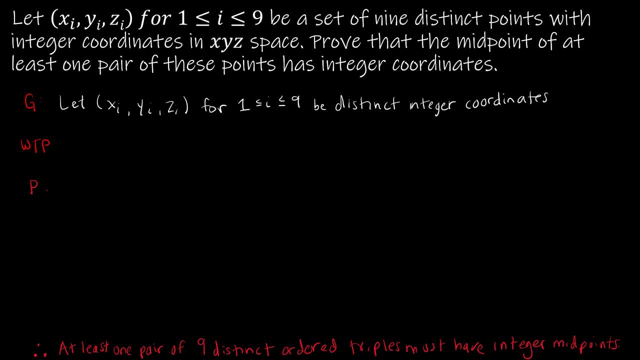 that at least one pair of nine distinct ordered triples must have integer midpoints, Or I went ahead and wrote how I was going to look at it in terms of finding the actual midpoint. So if you're familiar with any of this terminology or notation, 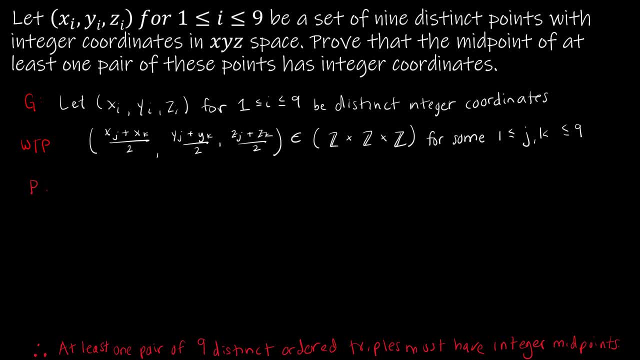 again, we were just taking x sub j plus x sub k, where j and k are between one and nine. So notice I didn't use i because i is just sort of the counting procedure. So I'm basically using j and k and saying these two values are between one and nine. 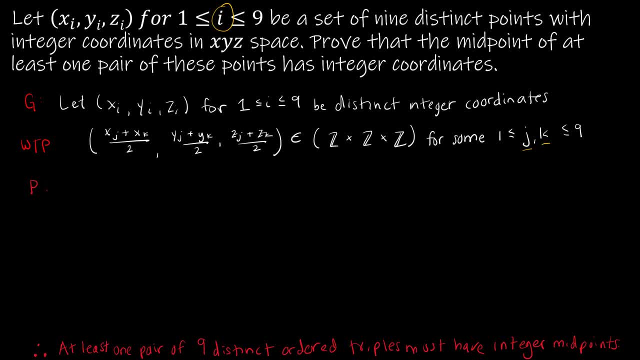 And I'm taking the x values and the y values from each. I'm taking the y values from each, I'm averaging them. So again, I'm basically saying I'm taking two points from this set and I'm going to find the midpoint, And I want them to be in the Cartesian product. 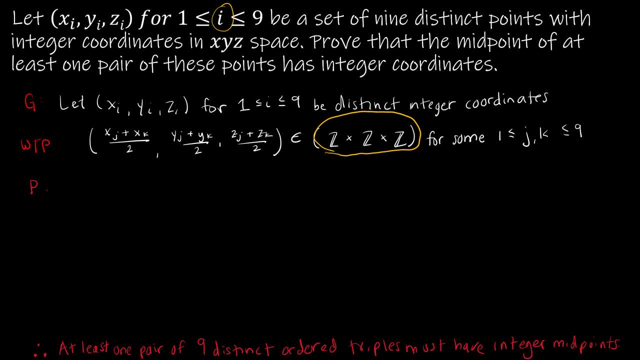 z cross z cross z, which just means the first value is an integer, the second is an integer and the third is an integer. So again, if that's confusing to you, you can write exactly what we have here. I just went ahead and wrote it out, particularly because it has that formula for. 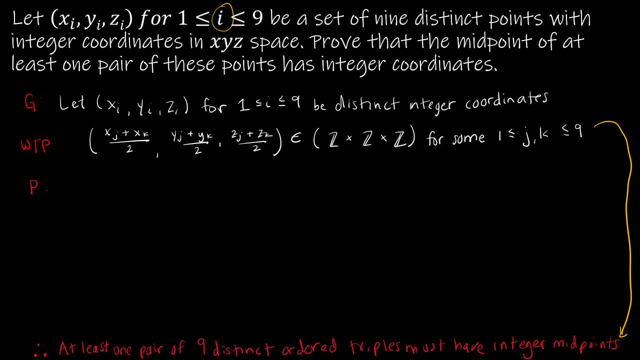 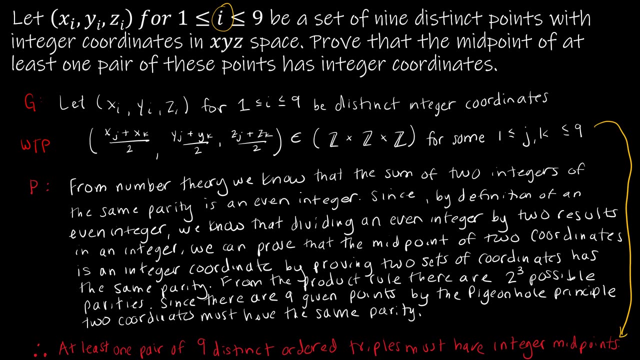 the midpoint in the what to proof. Now for the proof again. you cannot assume that whoever is reading your proof knows what we just talked about on the last slide. So, as I'm starting my proof, and the reason that I'm just showing you the proof as opposed to say writing it out as we go, is 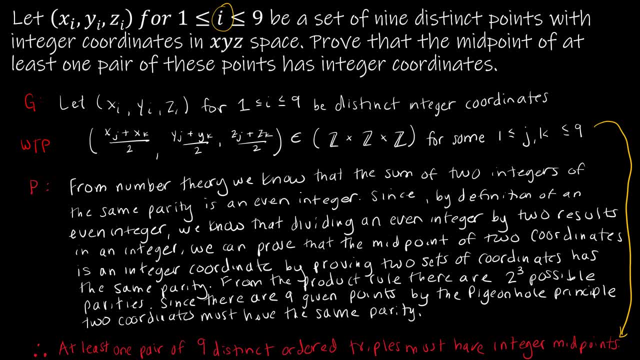 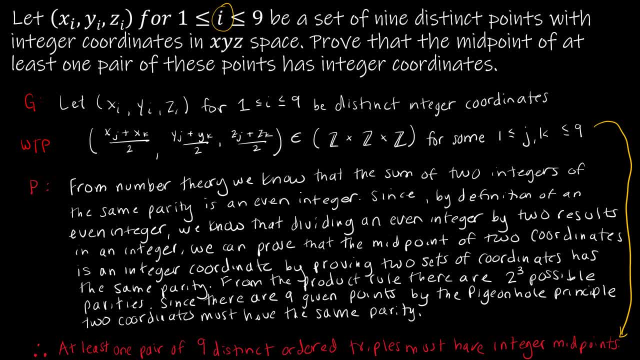 going to do that, So I went ahead and wrote it out. But again, I'm just kind of saying what we did on the last slide. From number theory we know that the sum of two integers of the same parity is an even integer, since, by definition of an even integer, we know that dividing an even integer by 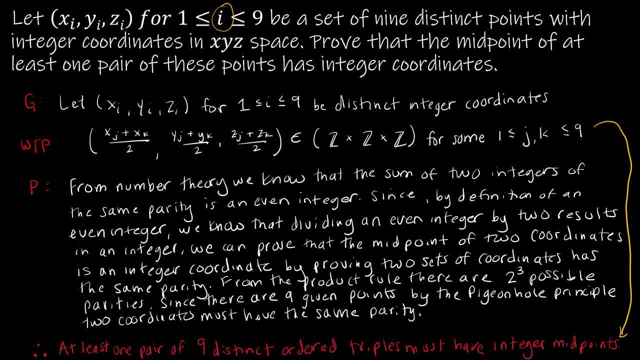 two results in an integer. we can prove the midpoint of two coordinates is an integer coordinate by proving two sets of coordinates have the same parity. So again we're looking for two integer coordinates that have the same parity. So again we're looking for two. 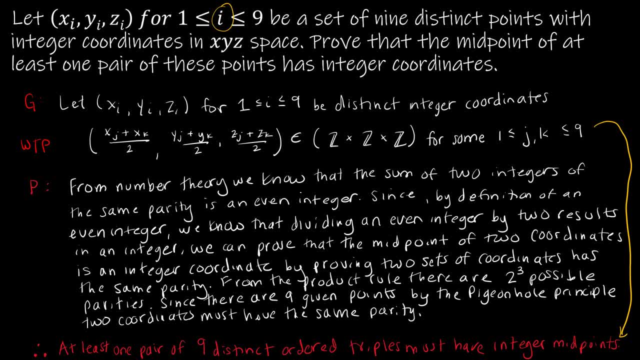 And what I'm talking about here, what I'm talking about the parity is. I'm talking about, say, even, even, even, and another one that's even, even, even, or two that have even, odd, even, or two that have odd, odd, odd. We get the idea We need them to have the same parity. 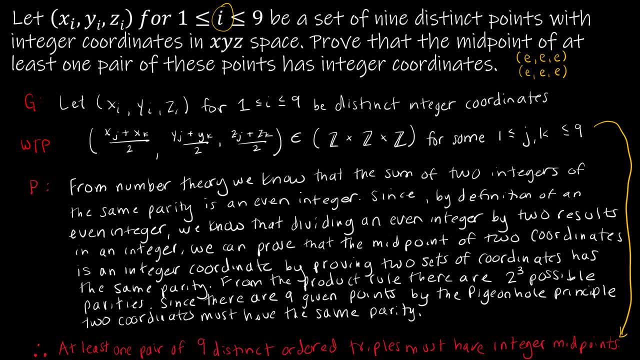 So, from the product rule, there are two to the third possible parities. So how do I know that? Well, because the first value can be even or odd, so that's two options. The second value can be even or odd, which is two options, And the third value is even or odd, which is two options. So I have two times two times two or two to the third, which is eight parities. 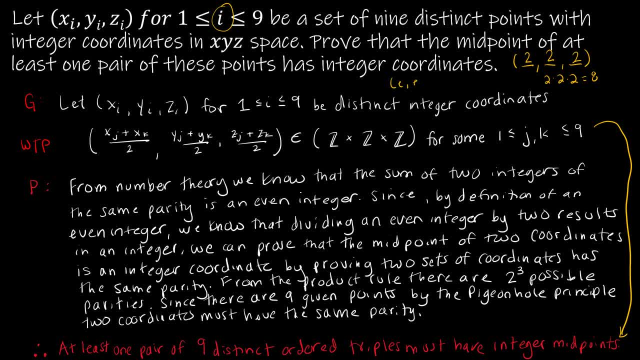 Now, what are those parities? Again, I could have, even, even. even. I could have odd, Odd, odd. Oops, I actually spelled the word odd, Odd, odd, odd. I could have, even, odd, even. You get the idea. There's eight of them. I'm not going to list them all out.